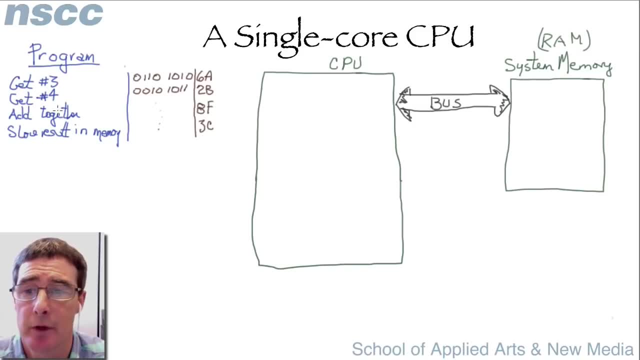 number three gets a number four, adds those numbers together and stores the results in memory. Every program, every step of a program, is converted to what's called an instruction. Now instructions in computers all have a binary code. So here's an instruction, and 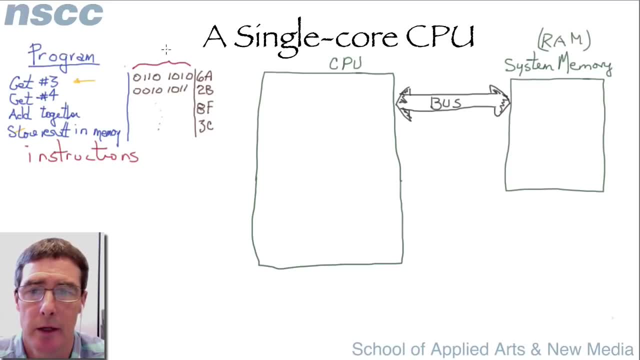 they're all unique to the CPU. So if you had a Pentium CPU, a Get 3 instruction would have a certain binary code, But if you were using a totally different, like an ARM CPU, could have a totally different binary code. And all these codes they're called the instruction set. So all these 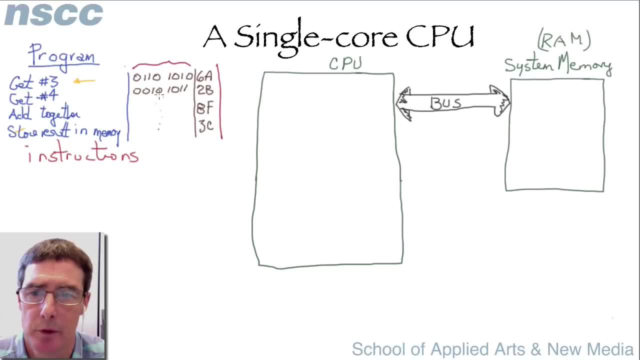 codes are in binary, but often people don't work very well with zeros and ones. We often shorthand this and write binary as a hexadecimal number, just because it's easier for us to to manipulate and talk about. Now the basic CPU system or computer system has a CPU at its center. 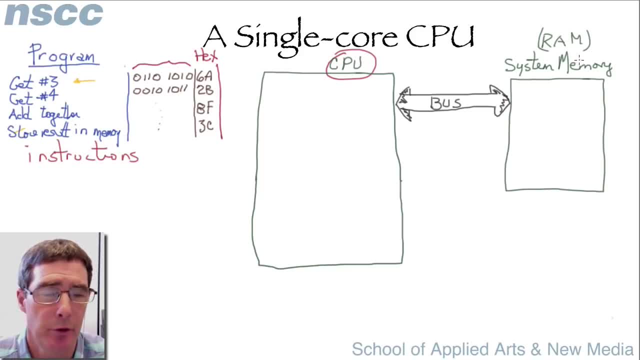 and system memory or RAM. For instance, in your personal computer you might have one gigabyte, two gigabyte, four gigabytes of system memory. Now, we're not talking about the hard disk or any optical disk. we're talking about the system, RAM And a. 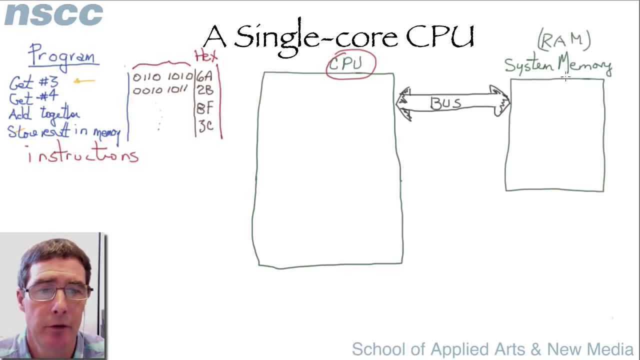 program or these binary codes have to reside in system memory in order to be executed. So somewhere in our system RAM we'll have this program that we want to execute. So if our program is on a hard drive, one of the first things that it has to do is transfer it to system. 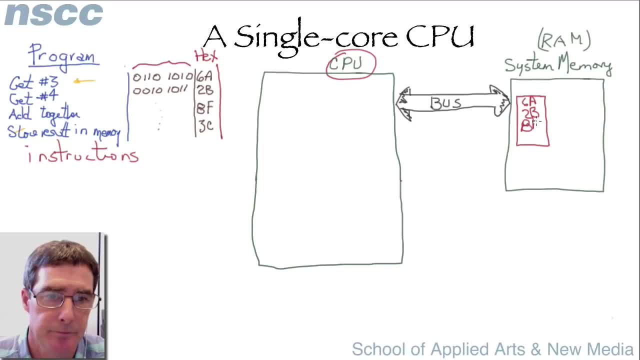 memory. Now that program is then read by the CPU, It's transferred to the CPU over one of the computer buses. There are many different types of buses- address and data buses and control buses- and they all work together. a lot of parallel lines to move. 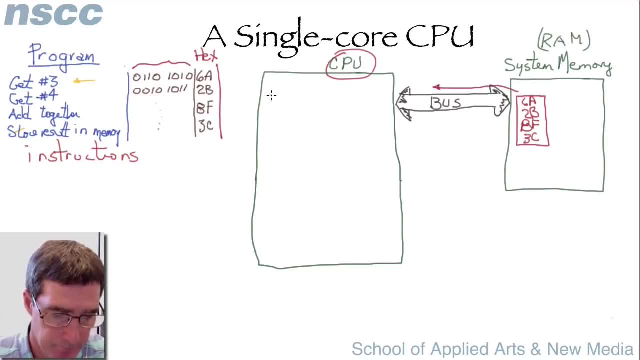 all these bits into the CPU at once. Now, once the program goes into a CPU, you can think of it as going down a long queue to be processed. So all these instructions work their way down this queue. So 3C was the last instruction. 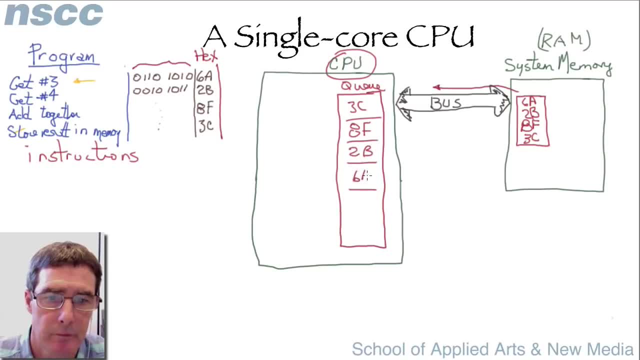 now this long queue is often given the name pipeline, And the CPU executes all these instructions using various components inside the CPU. So, for instance, we might have a math processor which will do adds and subtracts, some multiplies and so forth, And then we'll have this long. 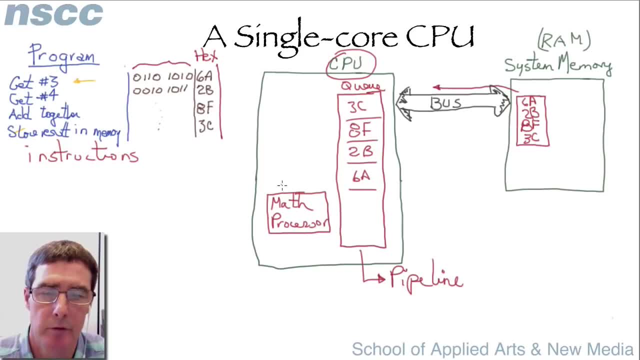 queue. Now this long queue is often given the name pipeline and the CPU executes all these instructions using various components inside the CPU. So, for instance, we might have a math processor which runs at다고 can even do scientific math, And we have multiple components which. 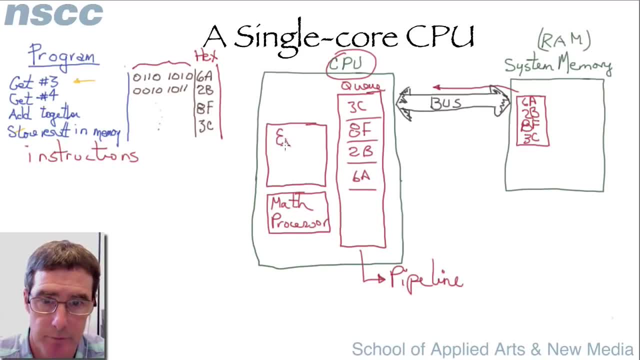 do some other parts, but we'll just call it the execution engine. And so what sort of is? the heartbeat for every CPU is a little clock that runs at a certain frequency. So, for instance, this clock might run at 2 gigahertz. 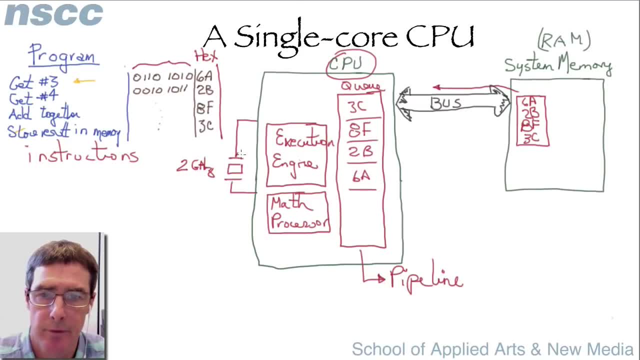 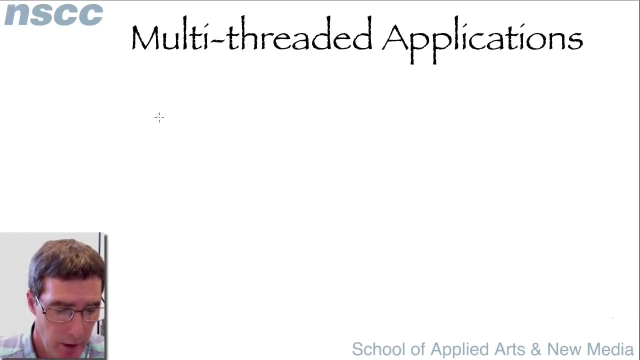 And it might go to various stages in the pipeline. Pipelines actually have stages before an instruction gets executed, But eventually it gets executed. So that's the basic operation of a CPU. Now we can think of this program as actually a thread. 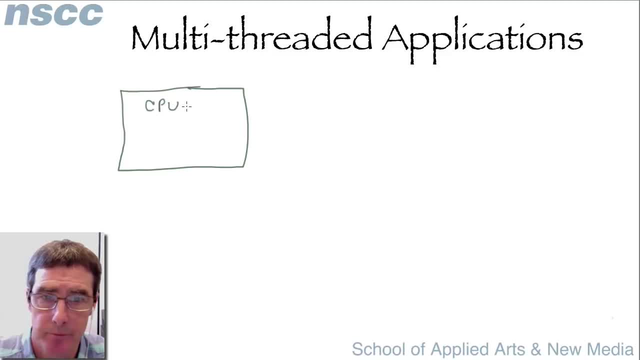 So if we have our CPU here and we have our program coming in as a bunch of instructions, And maybe these instructions are from an application And we'll use maybe Microsoft Office Word application As they come in, we can think of this as a unit of execution. 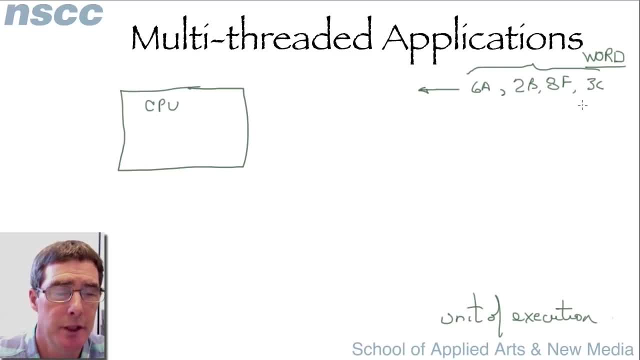 Which means it's a collection of instructions which together form some specific task And that's called a thread. So this thread is being read into our CPU. So here we have a thread And here we have a single-threaded application. 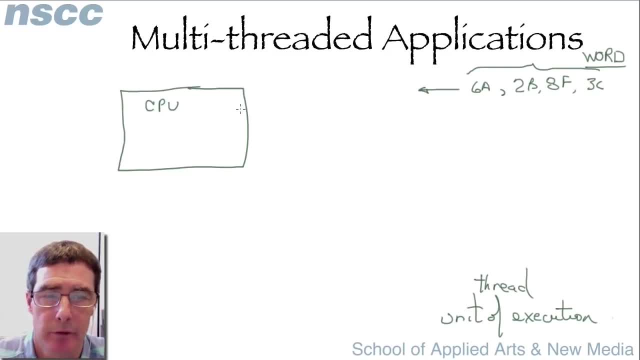 And that was how things worked in the days of MS-DOS and command-line-based operating systems. Very quickly, when Windows came in and Mac OS X, we quickly moved to a multitasking operating systems Where we wanted to have multiple applications open at once. 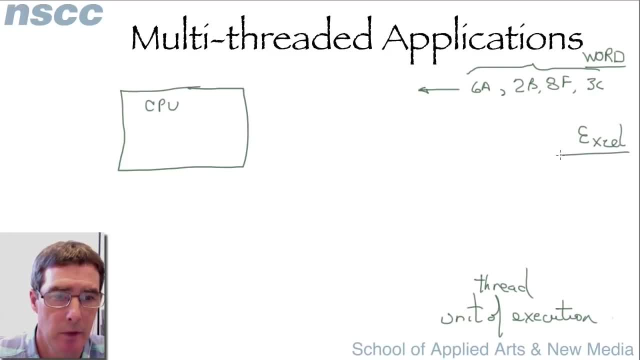 So we may have a second application, Maybe an Excel spreadsheet And it has its own set of instructions that are being executed to carry out its tasks. Maybe it's generating a recalculate on a spreadsheet, And so now we have a second thread that we want to execute. 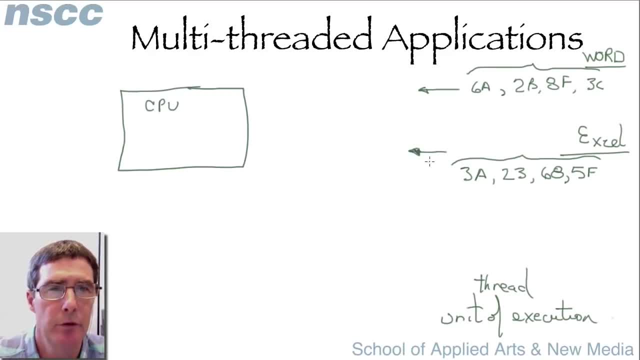 And we want it to appear to the user that it's being executed at the same time. So in all operating systems we're modified to introduce a new component in here And this component is called the scheduler, And it was a software component that basically controls these instructions getting to the CPU pipeline. 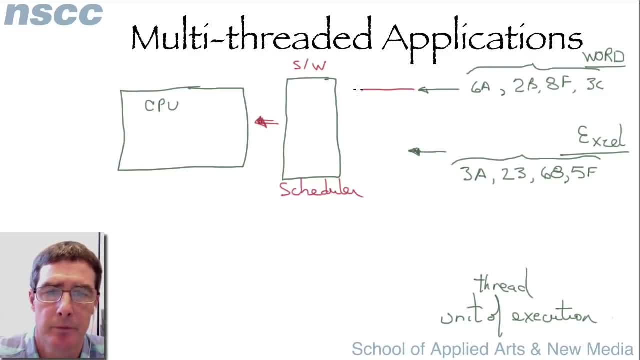 To be executed. So you can think of it in this case as having being able to handle the two threads And it really being just like a switch that can change positions from here to here And, depending on the position of the switch, if the switch is up here, this thread or these instructions go to the CPU to be executed. 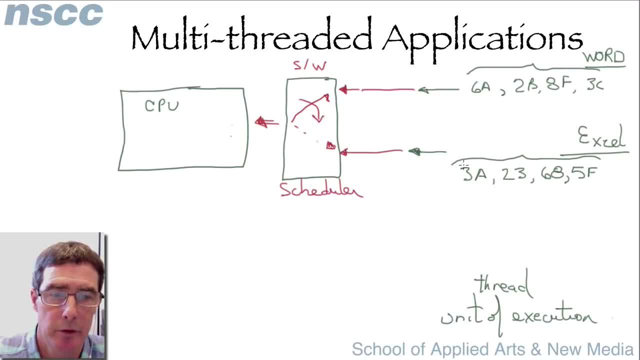 And this switch can change to the bottom position, And then this thread goes in to be executed. And this is what happens in today's multitasking operating system. Now, when this switches back and forth, it actually does so on a regular basis. 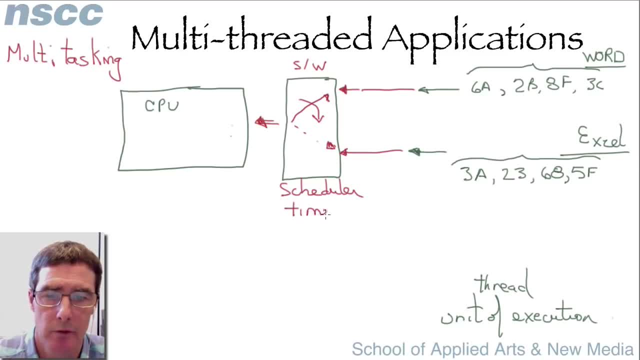 And that regular basis is called a time slice. So, for instance, maybe the time slice is one millisecond, So in one millisecond we could actually execute thousands of instructions from Word. And then we're going to switch over and we're going to execute thousands of instructions from Excel. 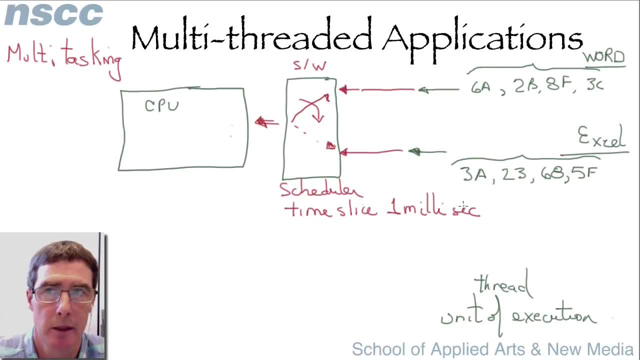 And we're going to switch back and forth every one millisecond. Now, as humans. to us this is going to happen so fast. it appears that everything is happening at the same time Or simultaneously. This type of multitasking is called preemptive. 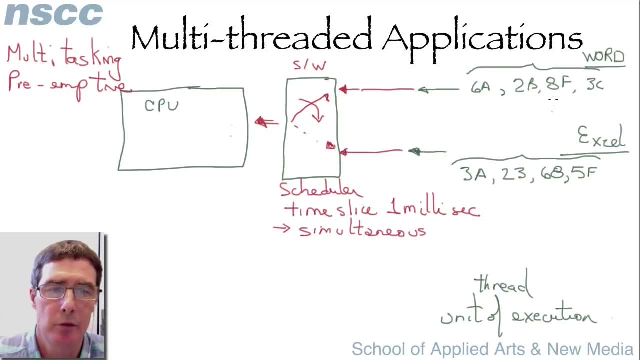 Preemptive multitasking, because it doesn't rely on any of these applications to give up control. This scheduler is simply going to take control away from one application and give it to another and work it back and forth. What's nice about that? If somehow Excel crashes, it's not going to crash your operating system. 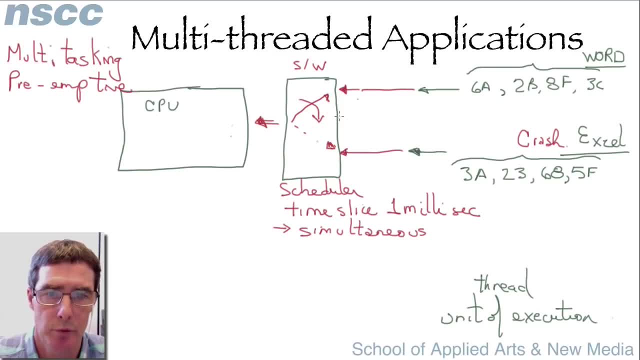 Yes, you may lose a time slice, but when you go back here, your Word program is going to work fine. And when you notice this is hung, you can actually just close it down by hitting the close button on your GUI. Now threads have other unique characteristics as well. 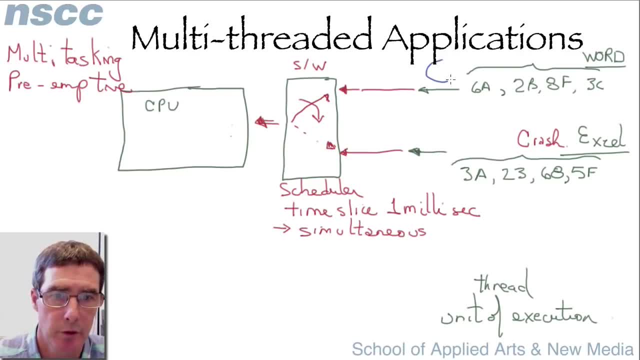 They also have something associated with them called a priority, And a priority is simply a number. Some systems use 1 to 32,, 1 to 99. So we'll say this has a priority of 10 and this has a priority of 2.. 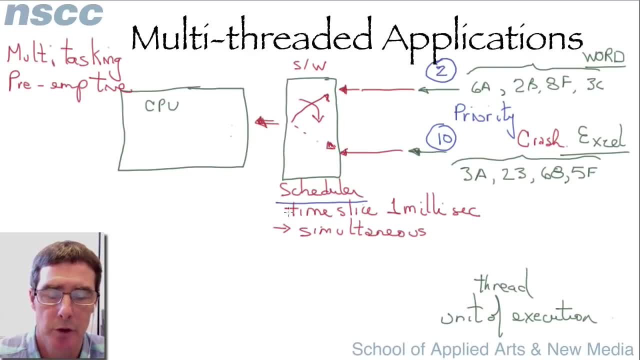 Now built into the scheduler. usually most schedulers simply give the highest priority thread a passage to the CPU. So what would happen here is this thread would give the highest priority thread And it would just stay in this thread because this is lower priority. 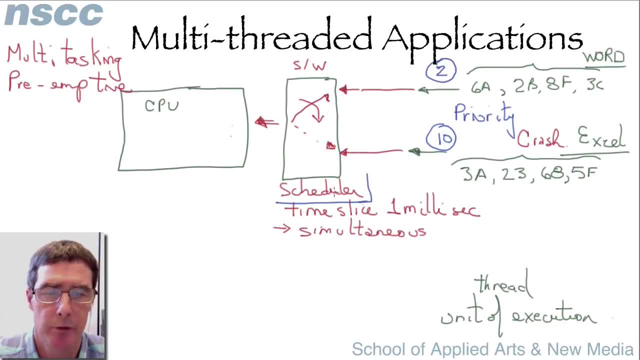 There's usually multiple parts to a scheduler And part of the scheduler's duty is to boost priorities of threads which don't get executed. So we'll go down here and we'll execute this thread for one or two time slices And then we'll boost this. 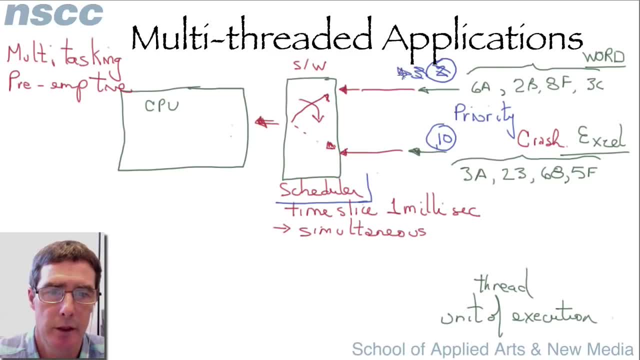 Execute Boost And eventually this thread will get up to the same level And then both threads will then what's called round robin: They'll both be executed a time slice until the thread's finished being executed. So this is how a multitasking operating system works. 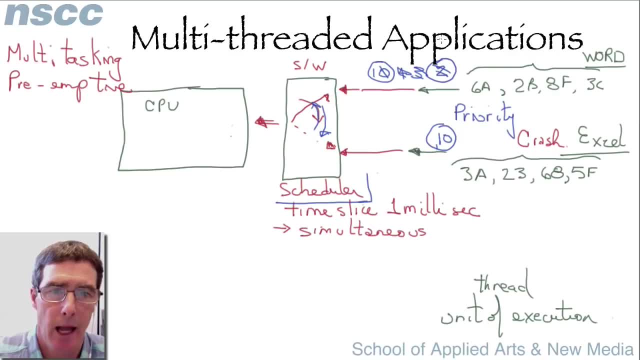 Now we talk here about multi-threaded applications, because most programs today- And so we're going to look at a program called Word And now we're going to call this a process- So a process is really a name for a program, But most programs today are multi-threaded. 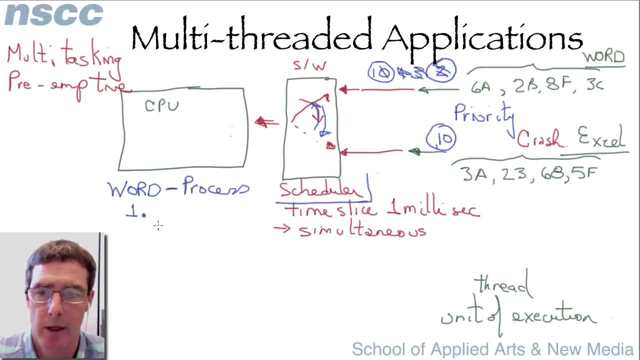 So, for instance, you may have one thread or unit of execution which is just looking for keyboard input, Waiting for the user to type something and then putting it on a screen. Maybe you've hit the print key But Or the print function. 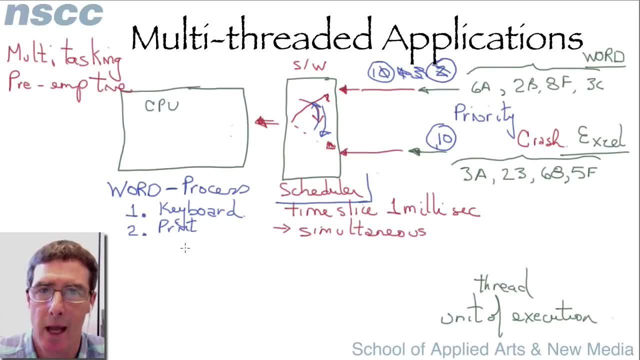 But when the print function happens, you don't want to wait for that print to be completed. You're going to get control back to your word processing program. So another thread is spawned, Another bunch of instructions are sent, or created and sent to the CPU which take care of printing in the background. 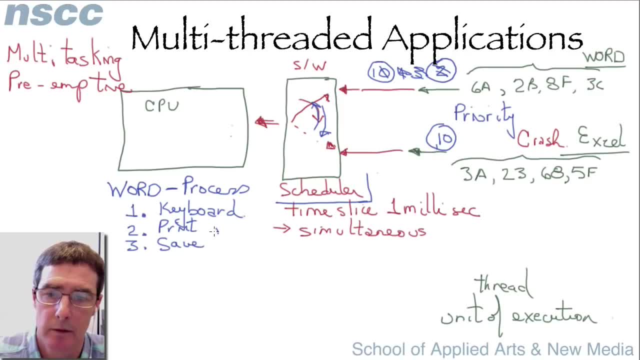 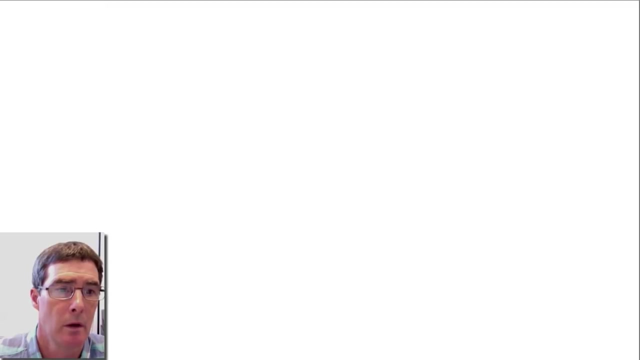 You may want to save a file That can spawn another thread. So most applications today are multi-threaded. Now today's CPUs Need to be different than they were 20 years ago Because we have these multi-threaded OSs. 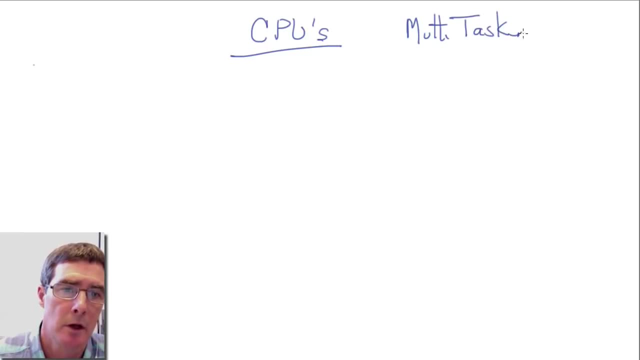 Multi-tasking OSs And we have multi-threaded applications. So today's CPUs are designed to be able to handle multiple threads more easily, And one of the first Systems was On a single CPU was Something called hyper-threading.